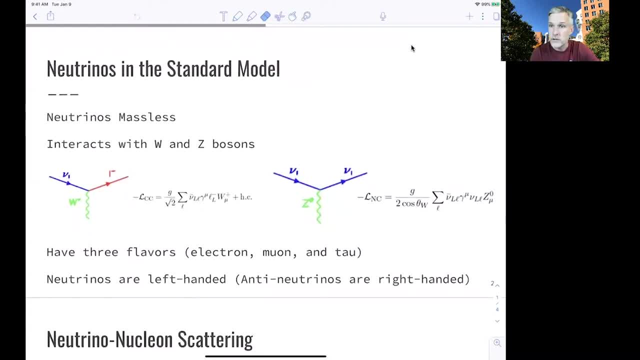 or try to write down the current, we find that there is a charged current via the W and there's a neutral current via the Z boson. It's quite interesting to think about those two currents. So in case of a charged current, if we, for example, have an incoming neutrino, we can 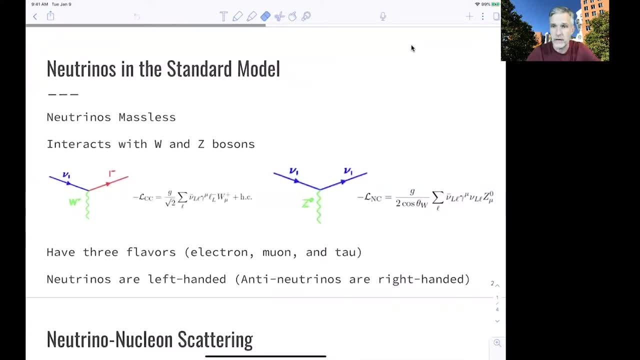 determine the flavor, the kind of neutrino we have. We are detecting the flavor of the lepton. So if we, for example, identify an electron in this interaction, then in the interaction the initial neutrino was an electron neutrino, While for the neutral current, when 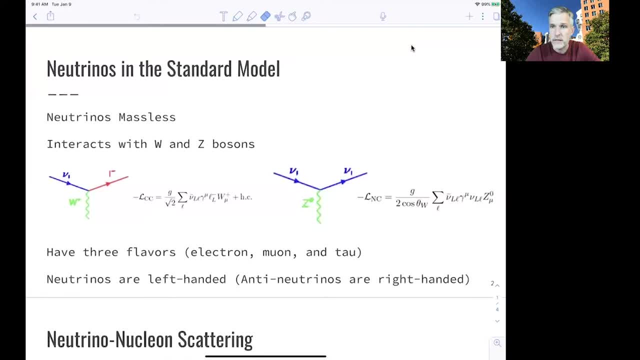 we have a charge current. we can determine the flavor of the lepton. So if we, for example, have some sort of interaction happening, we cannot identify directly the neutrino. Hence we cannot find the flavor of the neutrino. We can just measure the sum of all flavors. 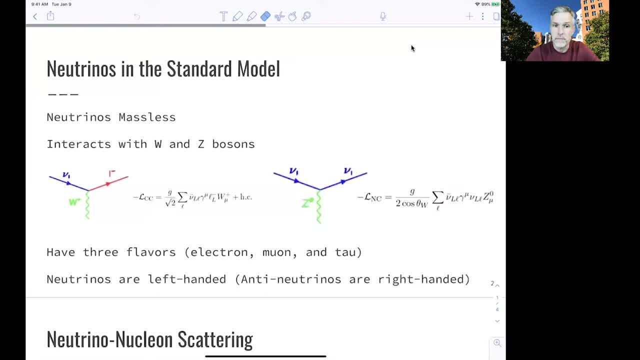 of the neutrinos in the neutral current. On that story. neutrinos have three flavors. They come in electron flavor, muon flavor or tau flavor. Neutrinos are left-handed, antineutrinos are right-handed. So that's the story. That's how neutrinos are characterized in the standard model. 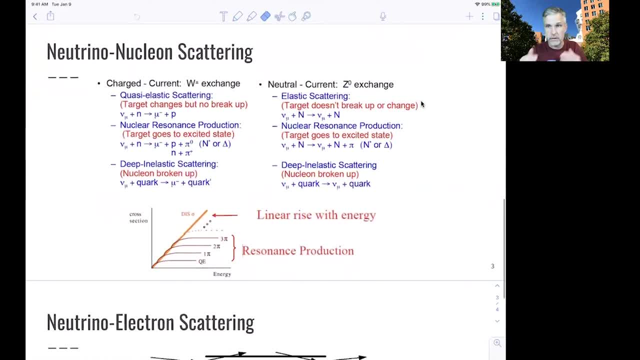 In the standard model, in the framework we set up, we can calculate cross-sections, scattering cross-sections, And here we are looking at neutrino-nuclei scattering Again. we can split this up in the charge, current and neutral, current discussion, but they go very much. 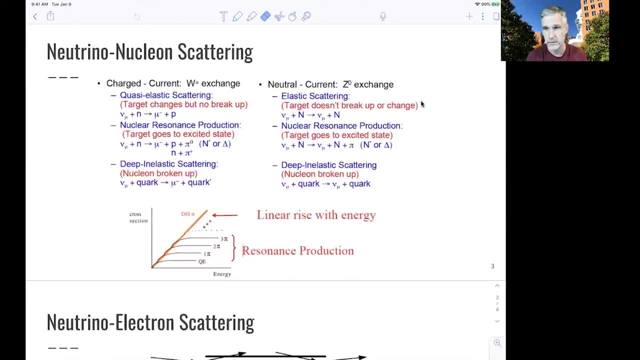 in parallel. So we have elastic scattering or, in the case of the charge current, we can talk about quasi-elastic scattering. We have an incoming neutrino, let's say a muon neutrino hitting a neutron, producing a muon and a proton. It's called quasi-elastic because 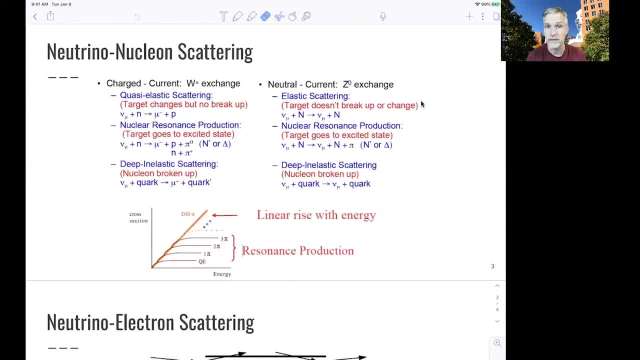 we do not break up the target, but we change its kind. So we change from a neutron to a proton in this case, While for the elastic scattering the neutron just stays intact. We can also have nuclear resonant production: we hit the nuclei and then inside the nuclei we produce a meson like a neutral or charged pion.